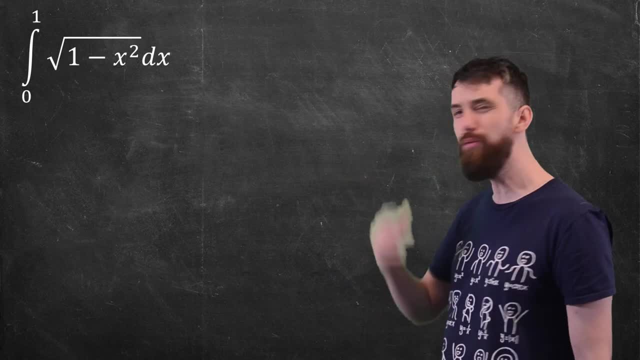 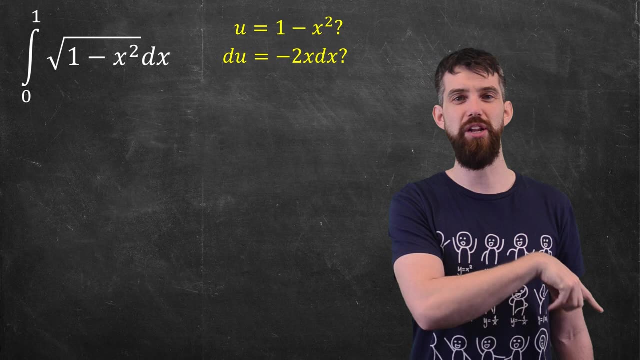 You might think we could do a u substitution like: oh, I don't know, it's a square root of blah. So what if we make that inside this one minus x, squared r u? But then our du is going to pick up. 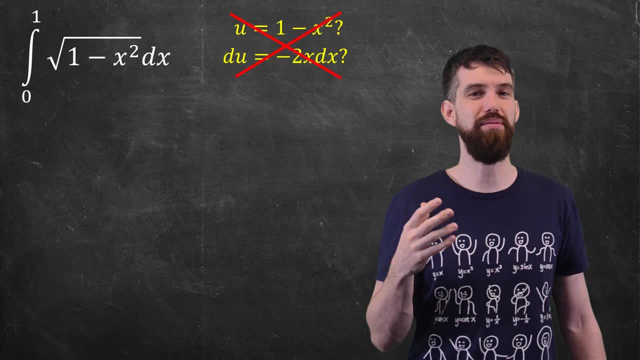 an x and there's no x outside of the square root, So it's going to be a square root of one minus x squared, and that just doesn't work out. Well, what else can we do? I'm going to do a different. 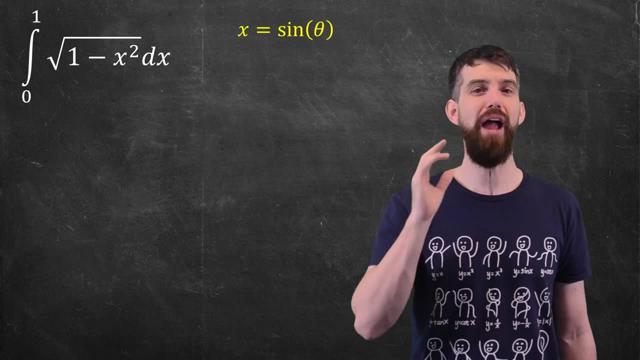 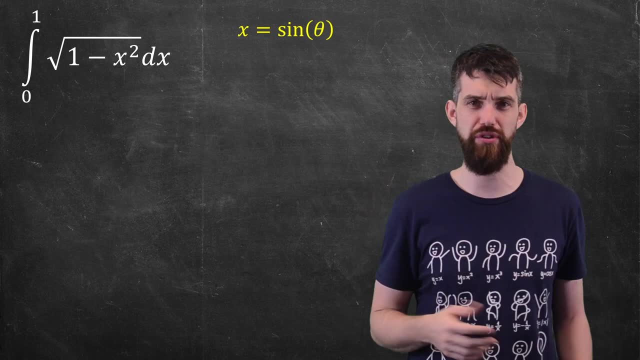 substitution. Just bear with me for a moment of why I'm choosing this. I'm going to choose a substitution. x is sine of theta. Notice that this sort of works in the reverse of how we normally do. u substitution: Normally we take some complicated, messy function of x and set it to be our new. 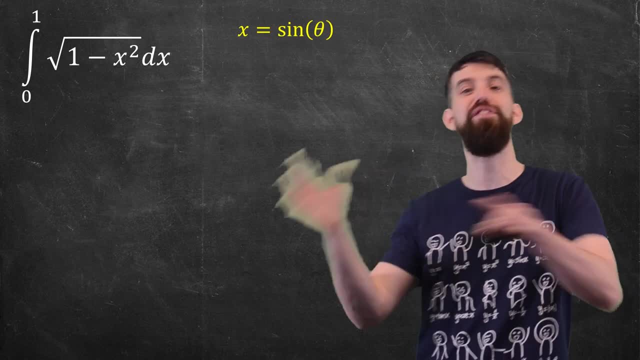 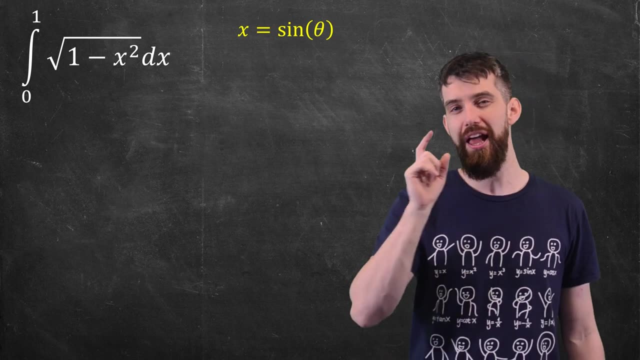 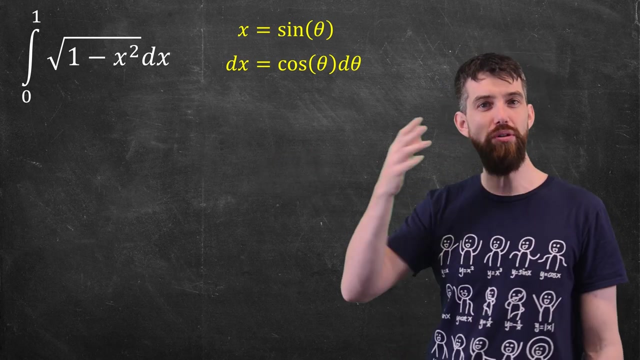 variable. Now we're taking the x itself and setting it to be some function of a new variable. It's sort of backwards for the normal u substitution, But nonetheless let's take the substitution and let's just see how it goes. This is our x. then our dx is cos of theta, d theta. And if I go to transform the integrand I also 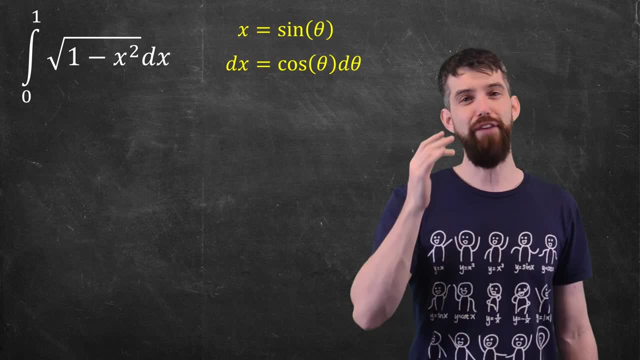 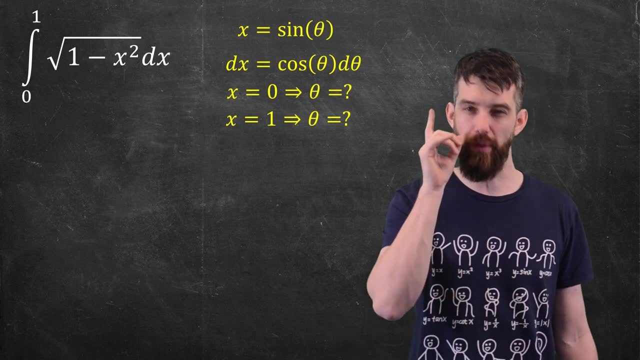 have to transform the limits of integration, the 0 and the 1.. So if I take the x equal to 0 or the x equal to 1, what theta value do I get out? Now there's a technicality here. There's a bit of a problem. 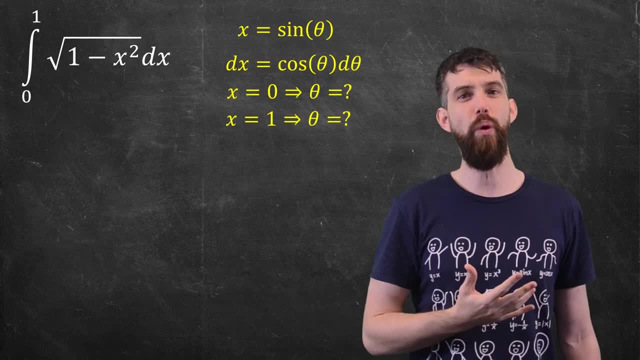 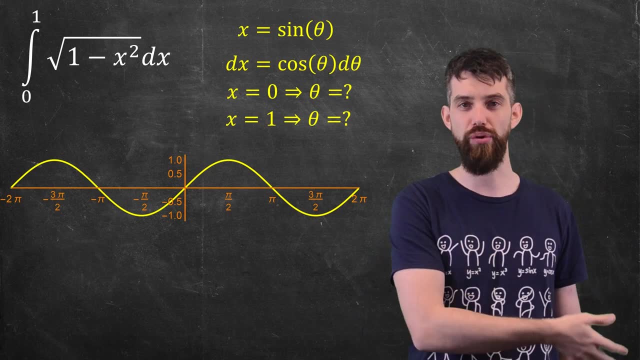 we have to work through because there's an ambiguity here. If you think about what the graph of sine of theta is, it's going to look like this. And if you ask: well, when sine of theta is 0,, what theta? 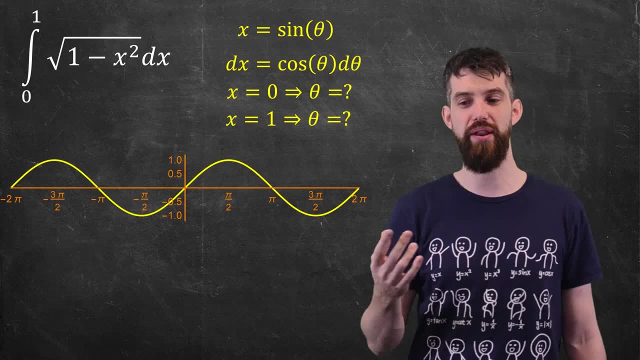 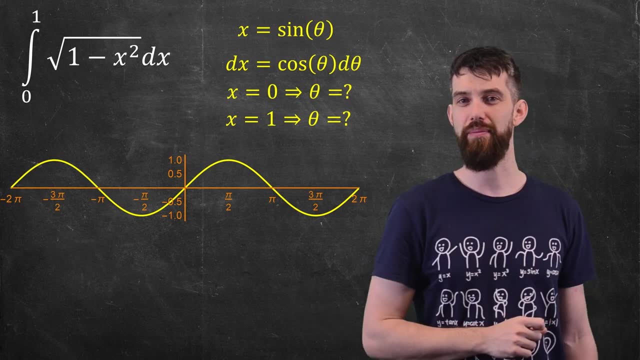 value is Well, sine of theta is 0 at theta equal to 0, pi 2 pi minus pi minus 2 pi, all sorts of places. So there's not just one answer here. Likewise for the value of 1.. Sine of theta is equal to 1 at pi. 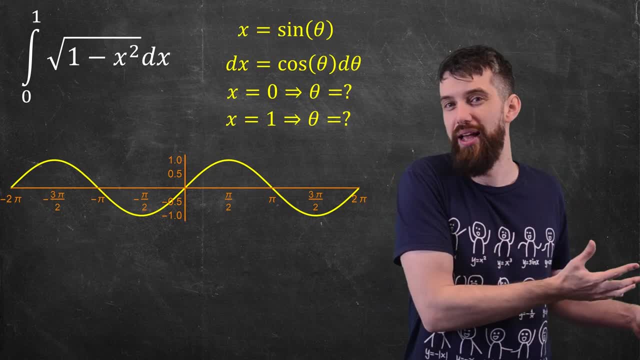 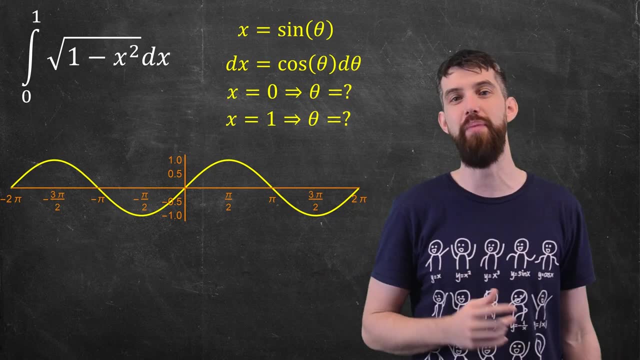 over 2, but also at minus 3 pi over 2, and many other values. So how do we resolve the ambiguity? I have to choose a region of sine of theta and restrict my domain to just that region that I'm going to talk about, For instance. let me take this region right here. 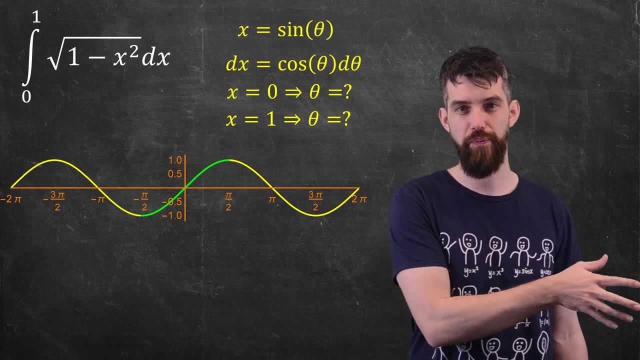 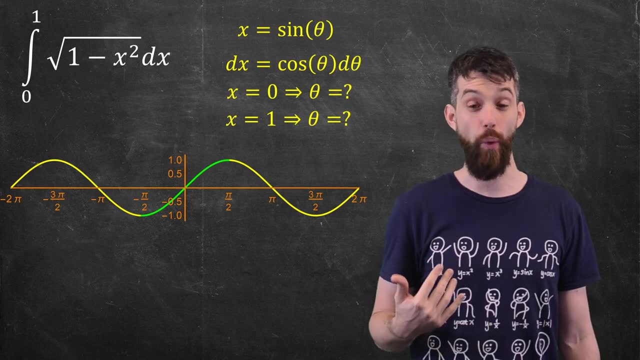 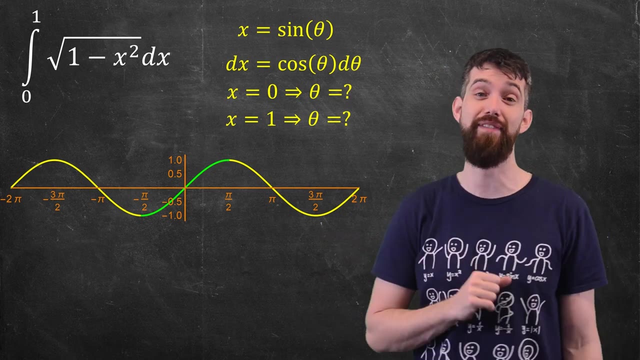 Notice that in this region the graph of sine theta. it attains all the values between minus and 1 and 1.. As in this region is big enough, Any possible value that sine theta could ever achieve is achieved by taking a value of theta between minus, pi over 2 and pi over 2.. But it's also achieved only once. 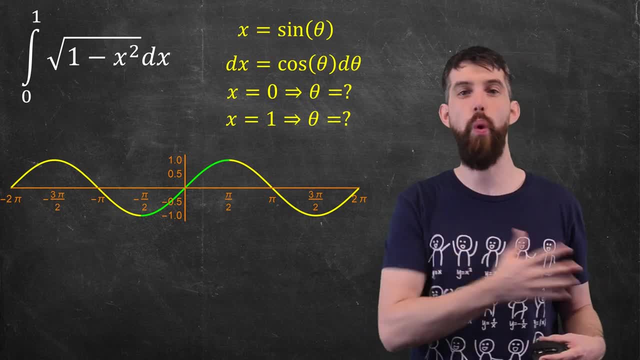 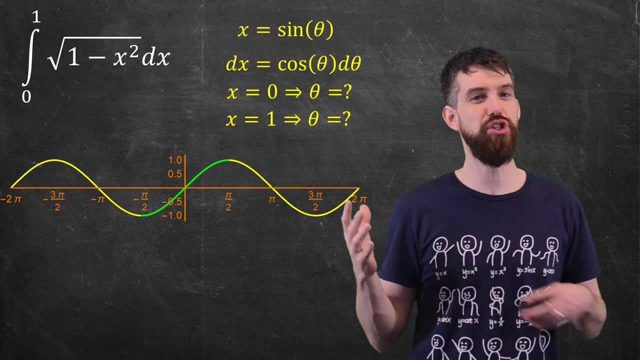 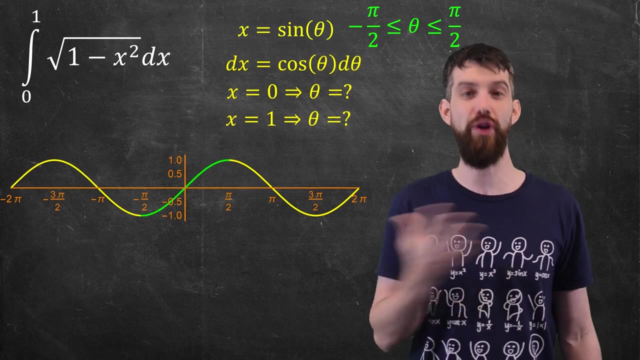 and that's the key idea. In mathematics we often call this 1 to 1, the notion that any value that is attained is only attained exactly once. But the idea is that if I restrict my domain to the green, to this minus pi over 2 up to pi over 2, then I can adjudicate questions like: if x. 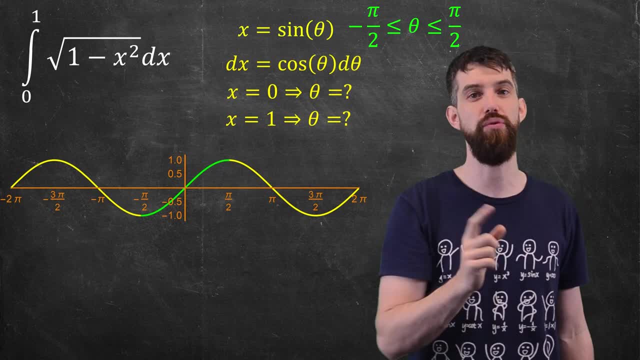 equal to 0, what value is sine of theta? and I can adjudicate them uniquely. So, in particular, if x is equal to 0, it forces it that theta is equal to 0. That is the only place where sine of. 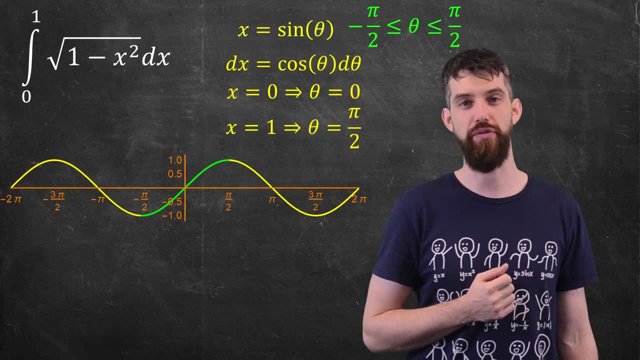 theta is equal to 0. And likewise for 1, it's going to occur at pi over 2.. So now that I've done all this sort of technical stuff, I can go on to the next one. So I'm going to take this. 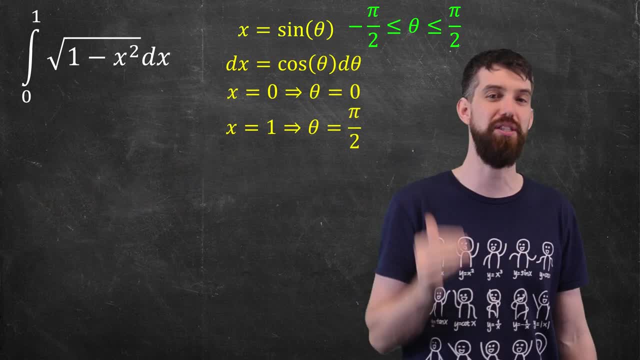 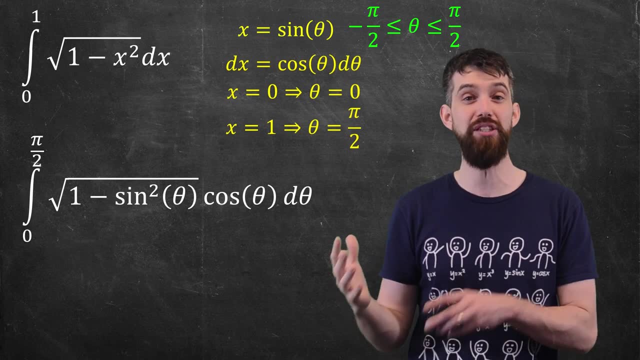 and plug everything in. I've got my x, I've got my dx and I've got my limits of integration. I plug those in and what do I get? 0 to pi over 2, the square root of 1 minus sine squared theta. 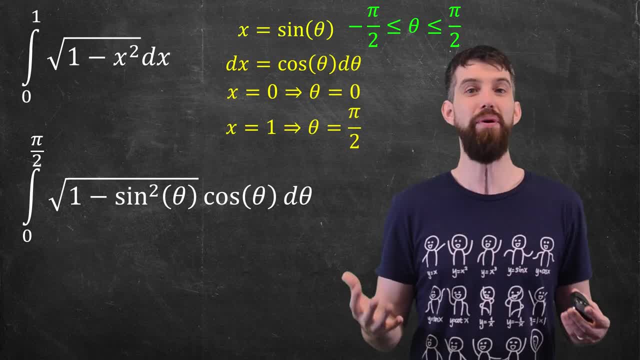 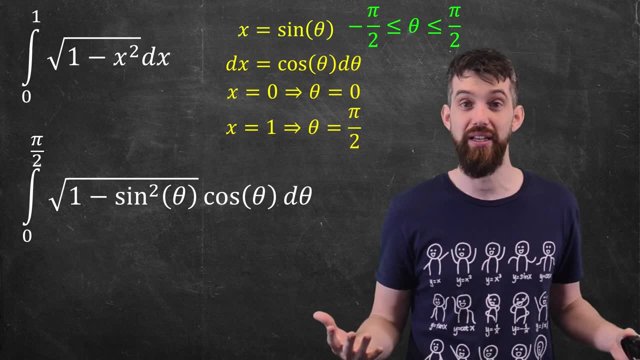 times cosine of theta, d theta. Now, what we've done is we've transformed this integral into 1, with a lot of trigonometric terms in it, And so what am I going to do? I'm going to use the methods of trigonometric integration that we've seen before. One of the things that stands out to me: 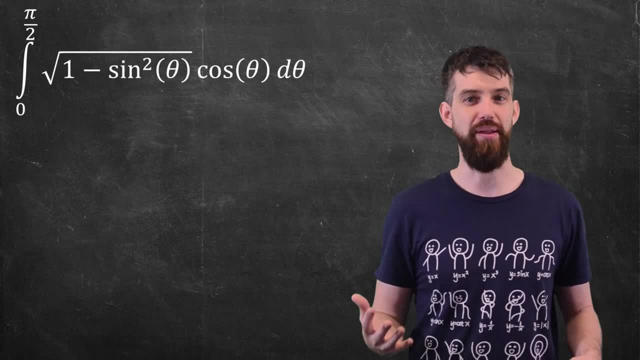 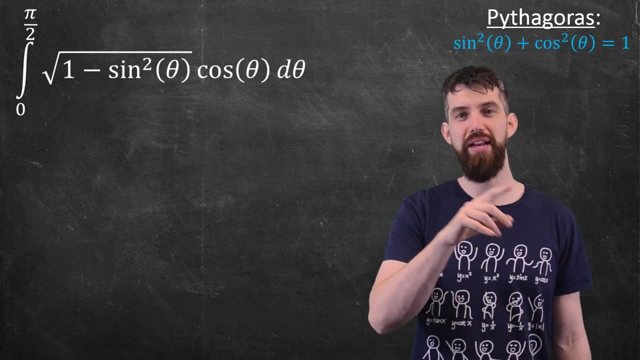 is the 1 minus sine squared, because I have an identity, I have that Pythagorean identity that sine squared plus cos squared is just 1.. And therefore, if I take the 1 minus the sine squared, that's going to get a cos squared inside of the square root. 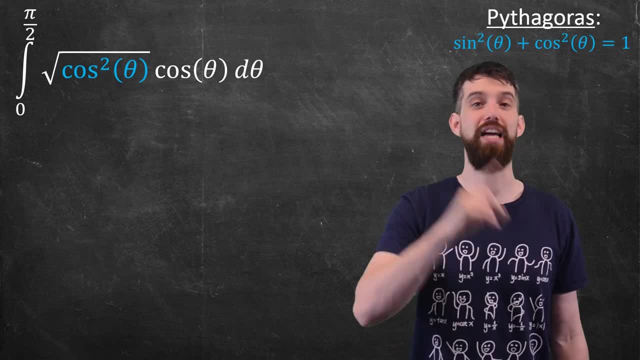 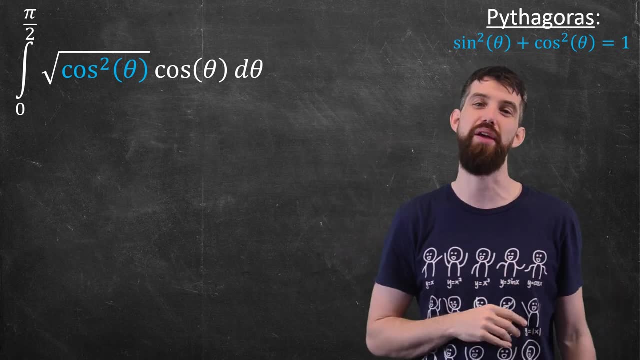 So I get the integral from 0 to pi over 2 of square root of cos. squared times another cosine of theta, finally the d theta. Now you might be tempted: square root of a square. Just write cosine there, Trevor, But you have to be careful about the sine, Because when I take the square root of something, 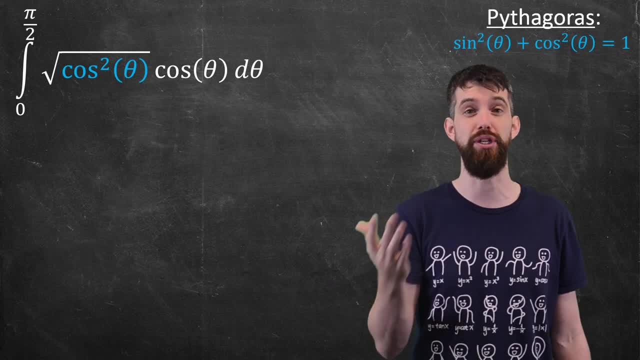 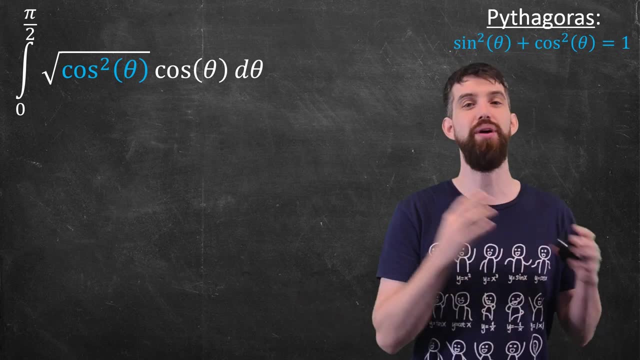 squared, I lose the plus or the minus. So it's pretty clear whether it's positive or negative. But thankfully I have that restriction on my domain. I know I'm talking about thetas between minus pi over 2 and pi over 2.. So if I look at what the graph of cosine was, 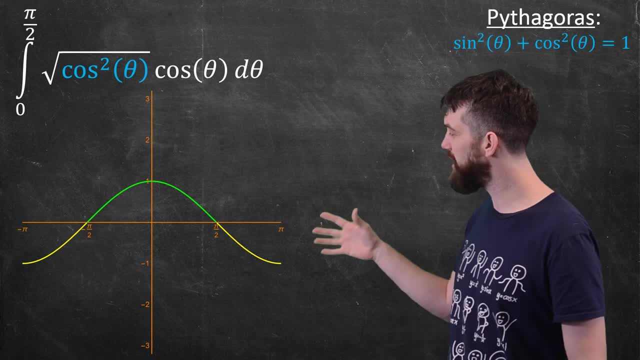 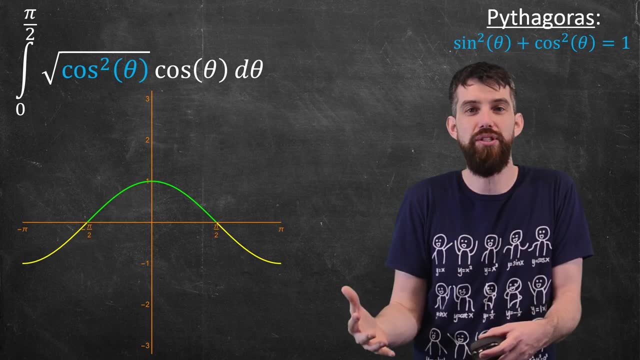 between minus pi over 2 and pi over 2,. you see how cosine is all positive in that green selection. So the square root of cos squared, it is just going to be cosine. There is no negative sign that needs to come in. 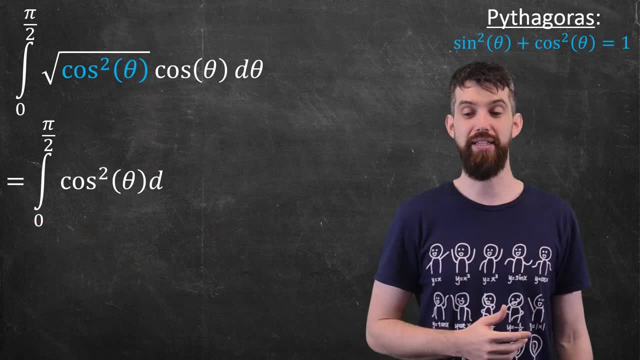 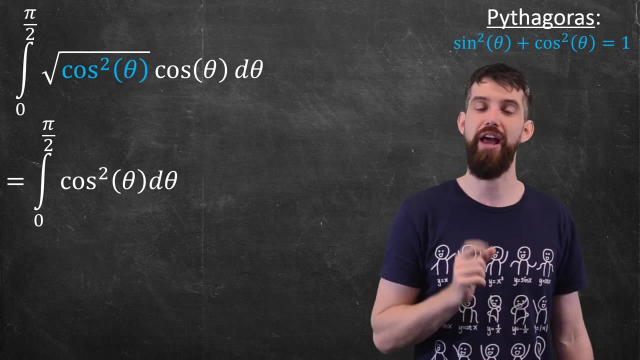 It's just all positive. So I can just replace this and say this is the integral from 0 to pi over 2 of 1 cosine, that's the square root of the cos, squared times another cosine of theta and then finally multiplied by the d theta. 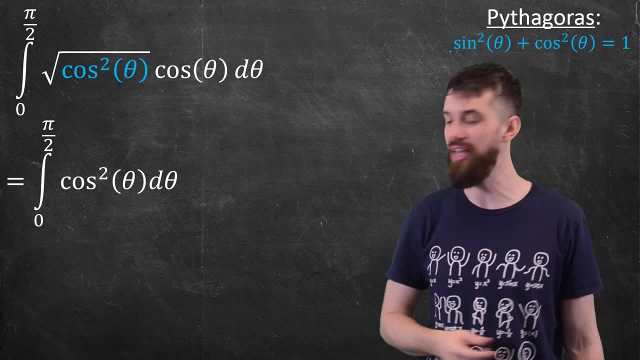 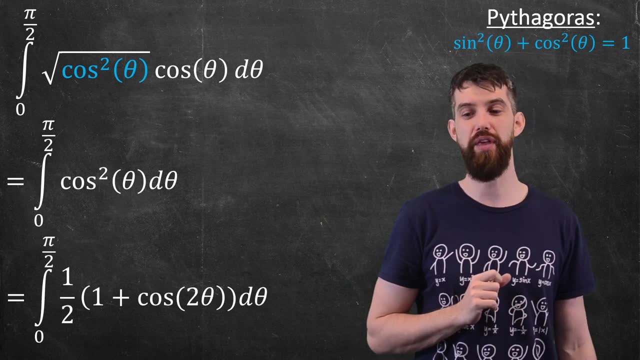 Now it's just a trigonometric integral. We can do the same method we've done previously. It's an even power, so we'll use that half angle identity. We rewrite that as one half of 1 plus cosine of 2, theta. 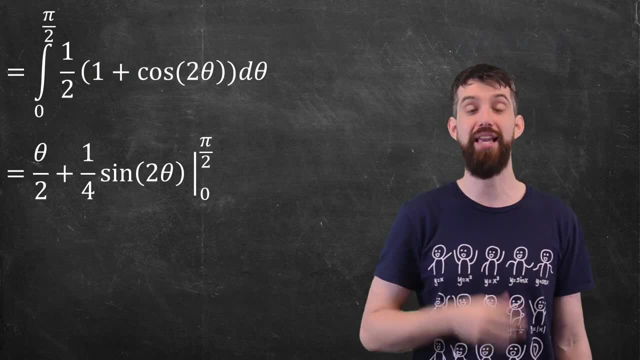 This is an integral that we're able to do, and so I can go and integrate that. I get theta over 2 minus one quarter sine of 2 theta. I evaluate between the 0 and the pi over 2, and voila, We get pi over 2.. 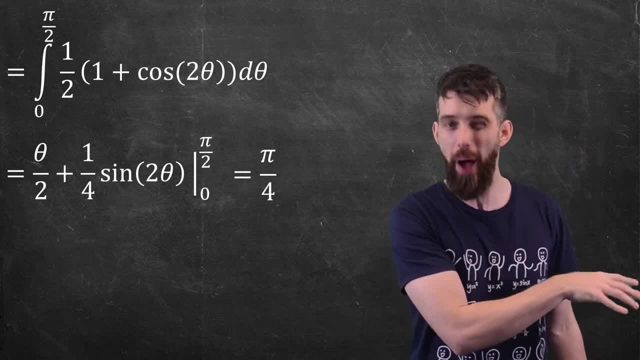 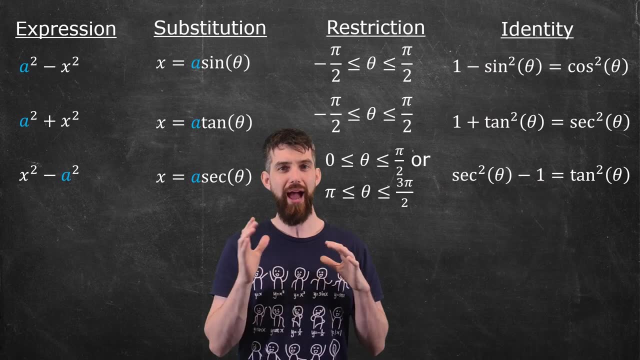 The answer that the area of a circle that pi r squared but we were doing a quarter circle. that answer was pi over 4 at the beginning and indeed we've got pi over 4 now. There actually is a bit of a chart for these kind of things. 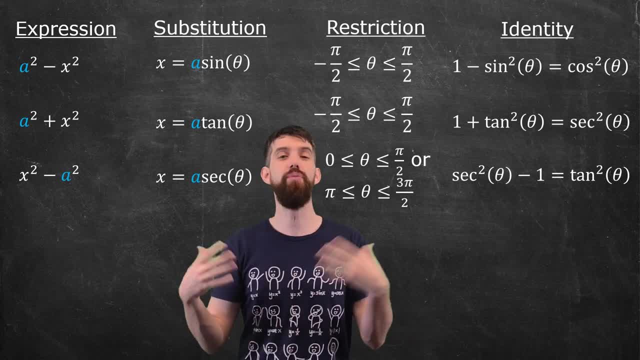 When we made that choice, that x was sine of theta. how did we do that? Well, I just gave it to you in this video. I didn't explain how. In the next video I'll talk a little bit more how to anticipate it. 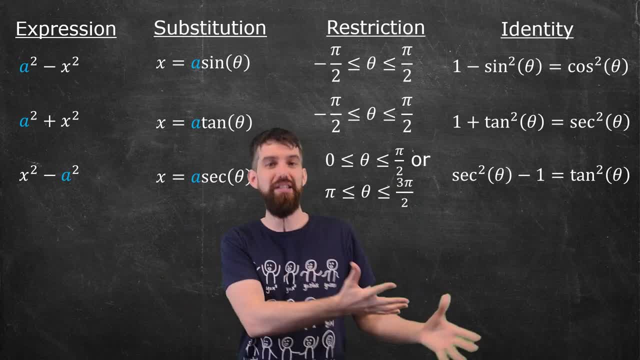 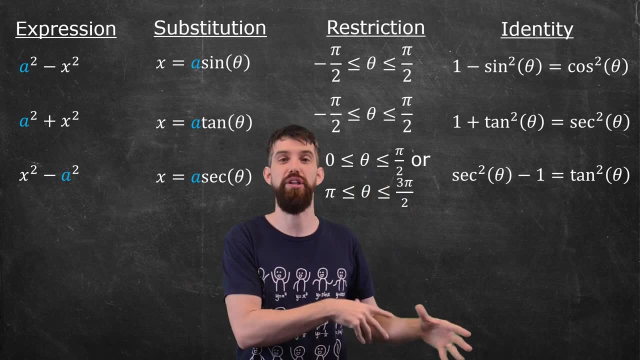 But, if you want, there is this chart here that tells you what substitution to use and what different situation. But, if you want, there is this chart here that tells you what substitution to use and what different situation, What the restriction on the domain ought to be and what trig identity you're going to use. 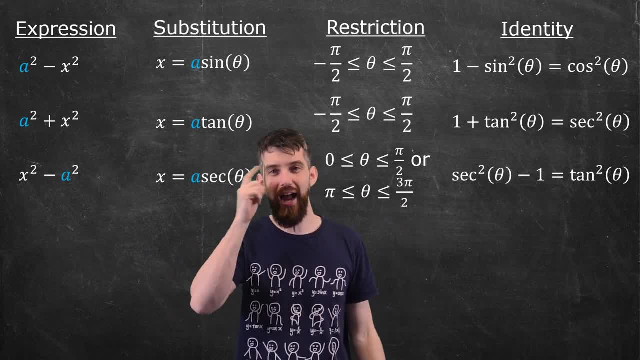 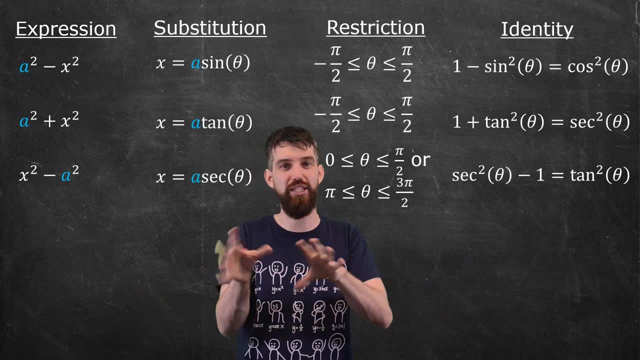 Now I'm putting this chart up here, but I would actually caution away from using it. I like to think through it, anticipating what trig identity am I going to use? What would be helpful if I had some expression? What should I try to do? Should it be sine cosine, tangent or whatever? 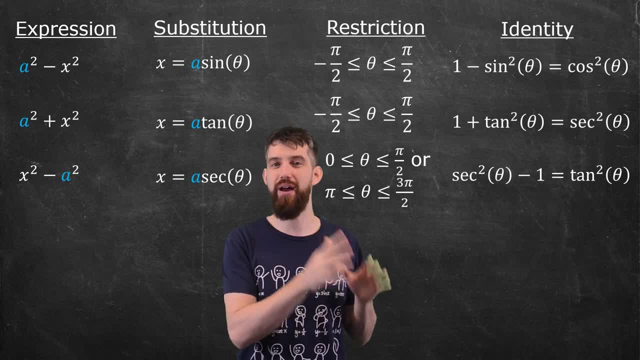 And I'll talk a little bit more in the next video about how to make those kind of choices. but here is this chart just to get you rolling.